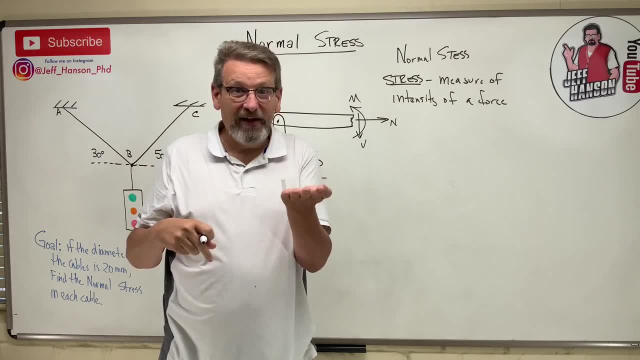 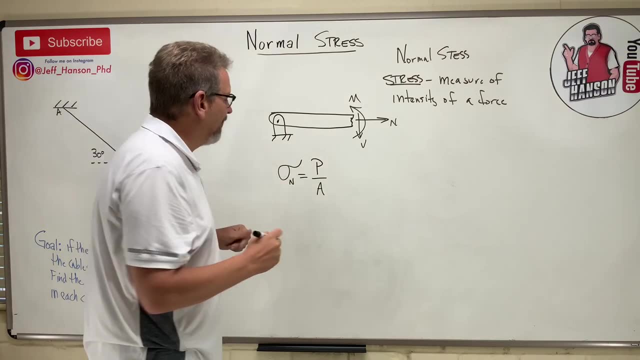 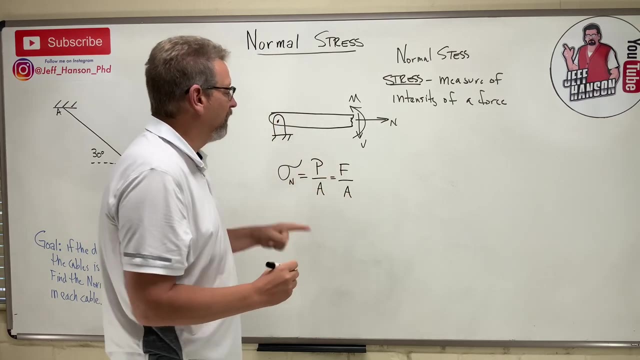 weight, right. The pain is very intense, The force is very intense. It's over a very small area. So we get this equation here: P over A. So what does that mean? Well, really, that's really force over area, right, Force over area. And if you really want to be specific, it's really the normal. 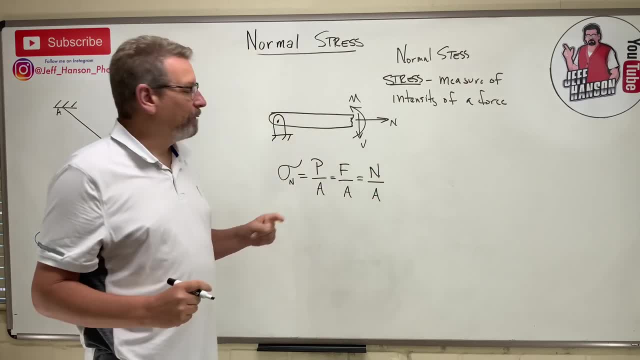 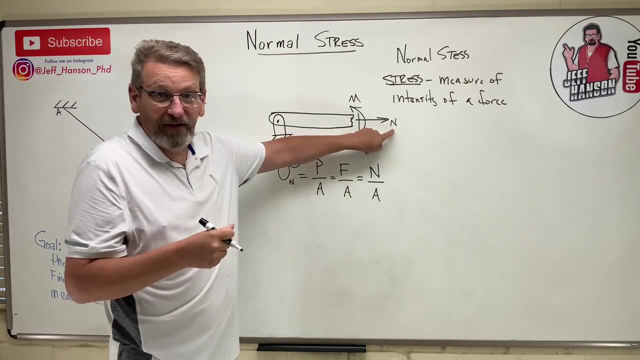 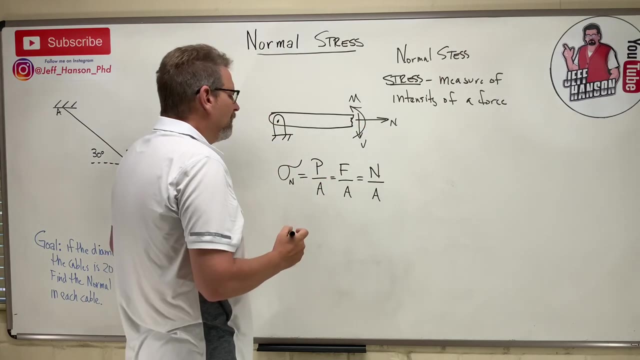 force over the area. okay, So P over A. you'll see it written P over A in the book, but it's a force over an area And that force is in that normal force, because that's the one that's either stretching you or compressing you. okay, And so what are the units for this? Let's talk. 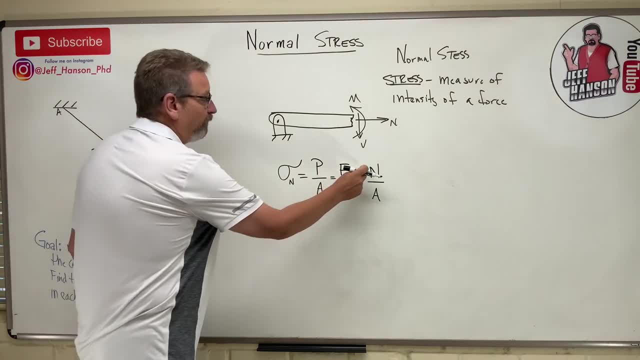 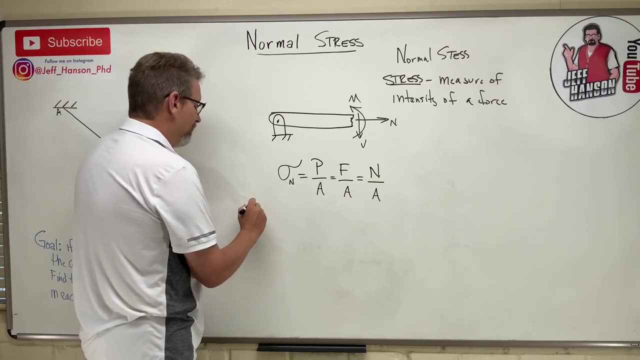 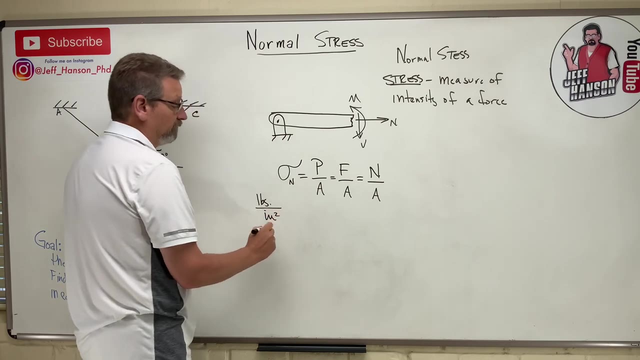 units for a second. The units would be something like: since it's force over an area in the English system in freedom, units right, P, S, S, S, S, S S S. something like pounds over inches squared, which is going to give you PSI right, Pounds per square. 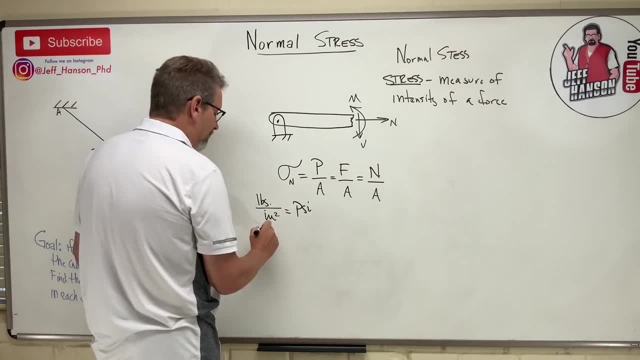 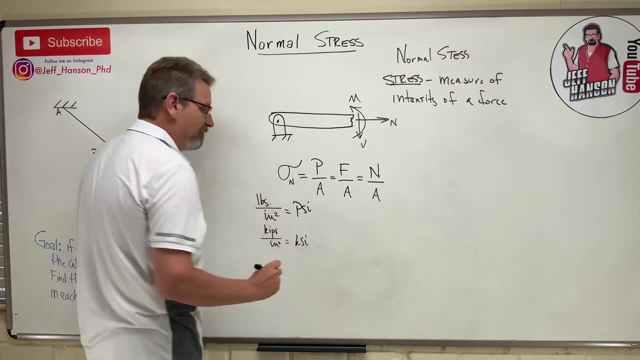 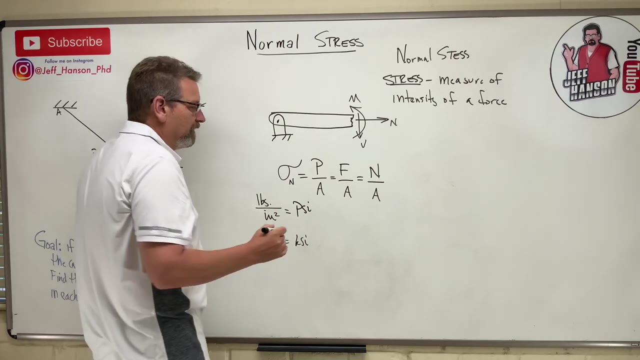 inch, Or you would get something like kips per inches squared, which is KSI. You might see KSI, that's kips per square inch, or kilopounds per square inch, whatever you want to call it. In the metric system, which is what we all should be using, I agree with you- is newtons. 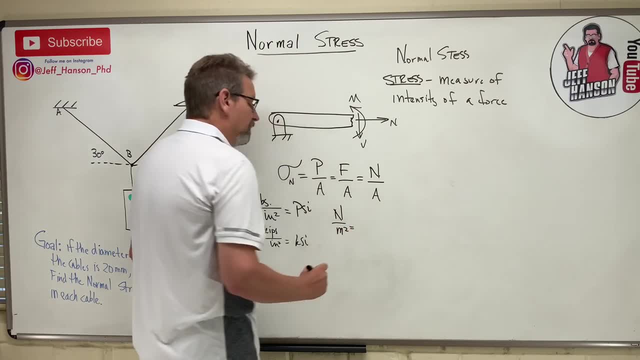 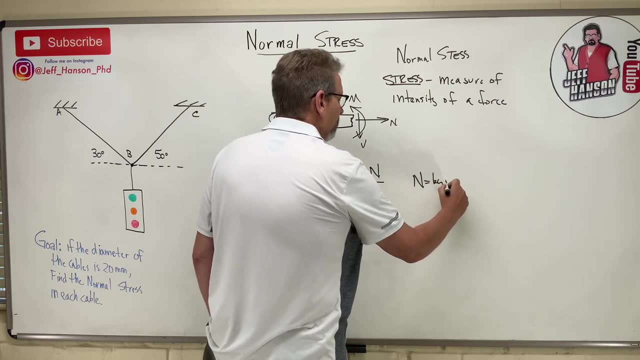 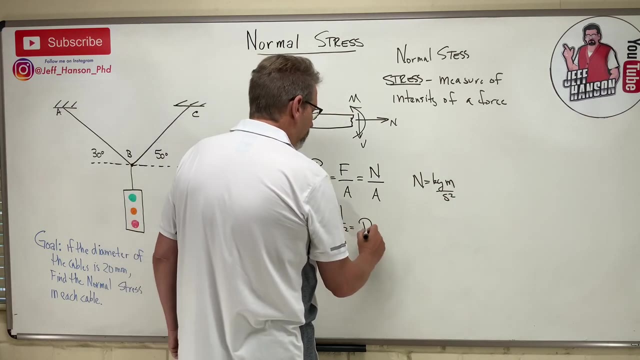 over meters squared. What is a newton over meters squared? What is a newton? Do you remember what a newton is? A newton is a kilogram meter per second squared right, And a newton over meters squared is a pascal, or you might call it a pascal okay. 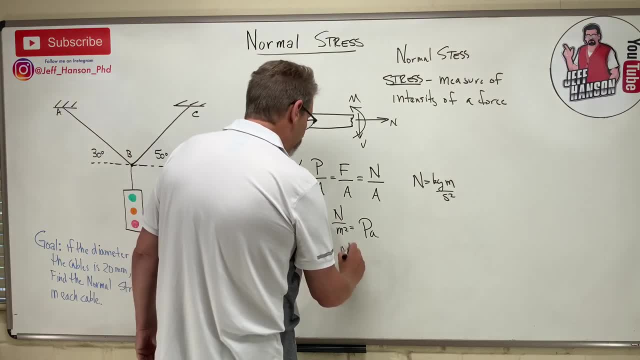 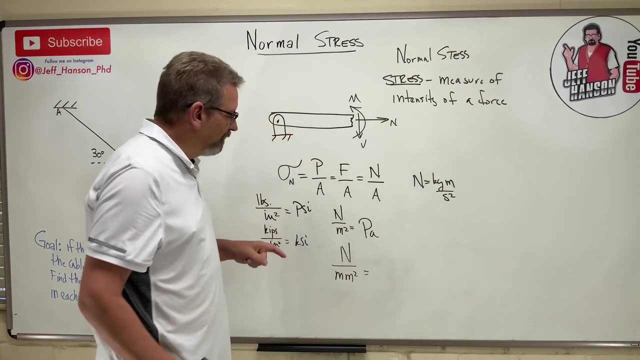 Then there's one more that's very commonly used, and that is this one. I like this one. This is my favorite one. okay, Newtons over millimeters squared- The way I remember this is newtons over meters squared is pascal. This one has an extra m on it, so where does the extra m go? 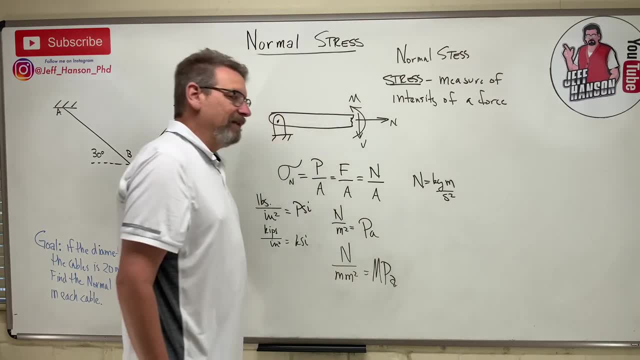 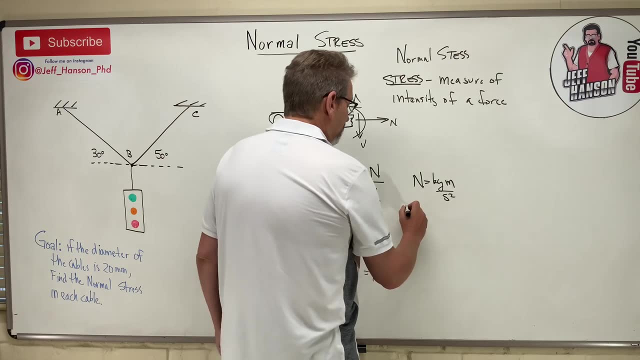 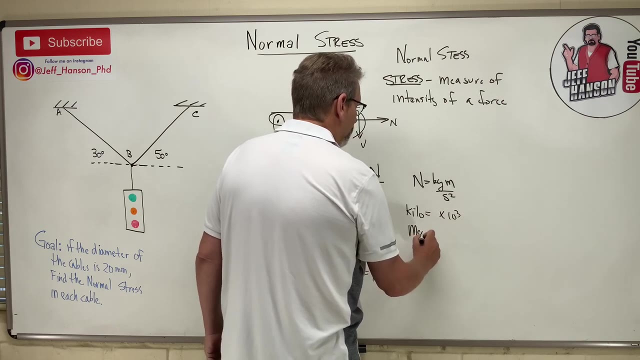 Right there in the front, okay, And that's a megapascal, okay. And the other thing that you really need to remember in solids, well, for anything really, is that kila right is times 10 to the 3, mega times 10 to the 6, and then giga whoa, times 10 to the 9,, right. 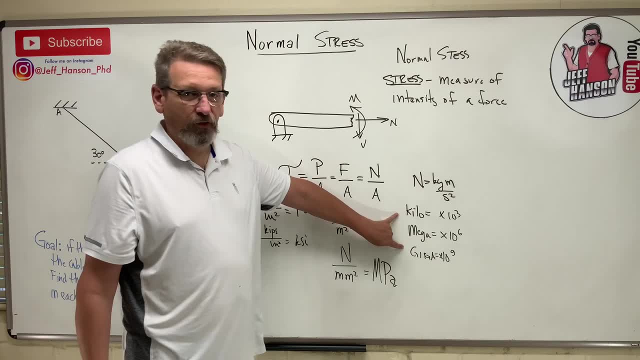 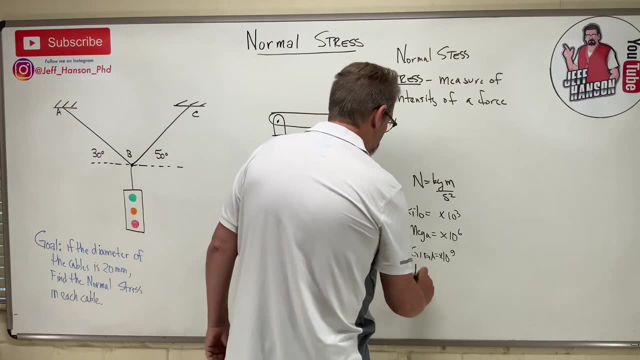 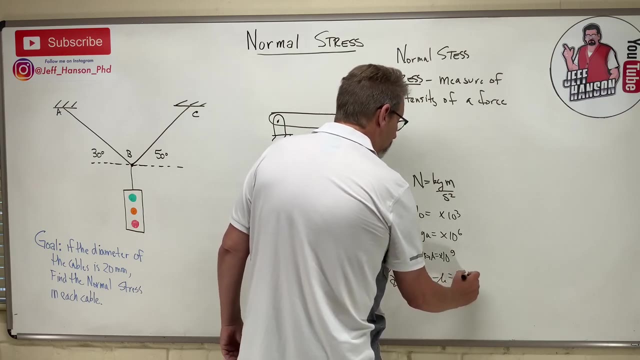 And then it goes on from there, But these are the ones you'll see most commonly in solids, And you also might see micro, right Micro, And micro is given with a mu, And that is times 10 to the negative 6, okay, So those are some things that you might see. 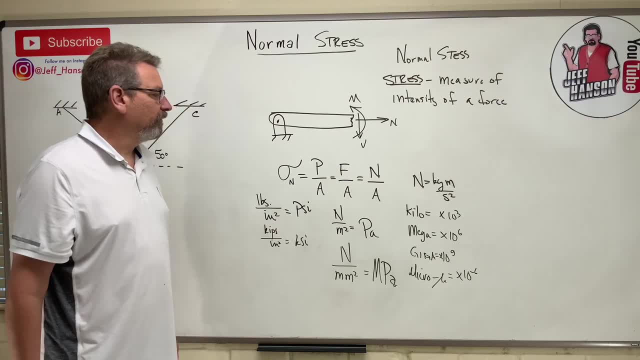 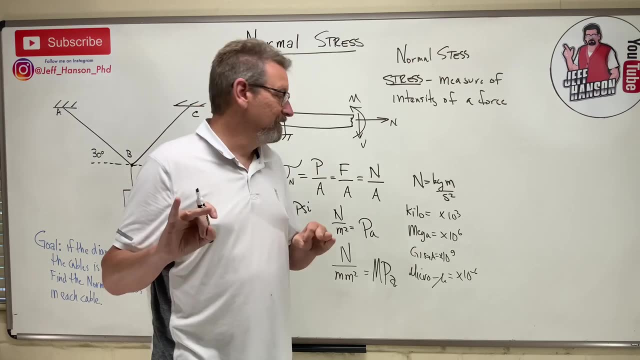 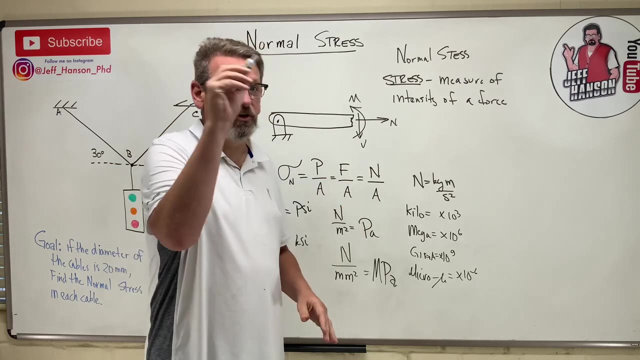 Those are just a little quick unit review for solids because in solids, if I had to say what is the number one thing to make me successful in solids- and it's real simple- it's pay attention and show your units right. Make sure all your units cross out. that this divides into that. 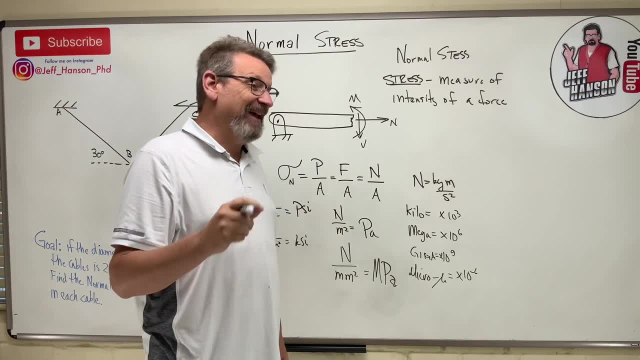 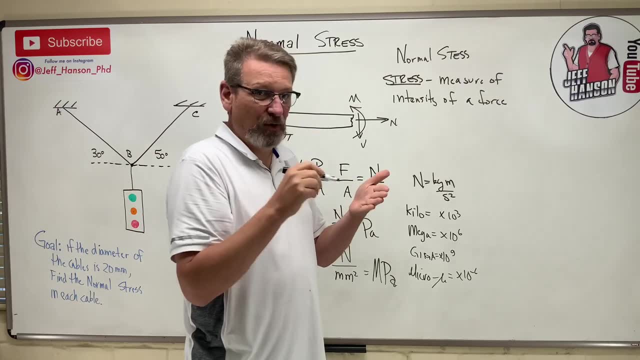 and that goes into that and that leaves me with: okay, I see, right, And show your units in your work, on your paper, not just on your answer, but in your work, And you'll see me doing this. I'll show my units, because is it 10 to the 3?? Is it 10 to the 6,? 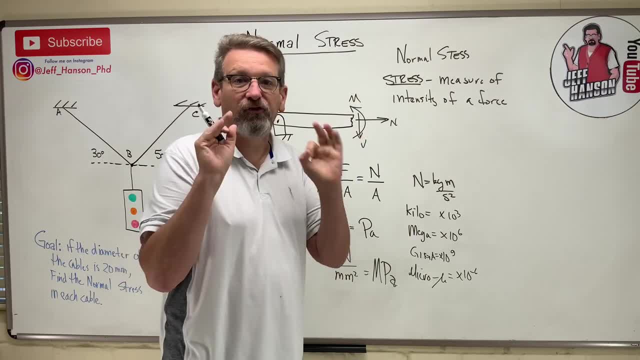 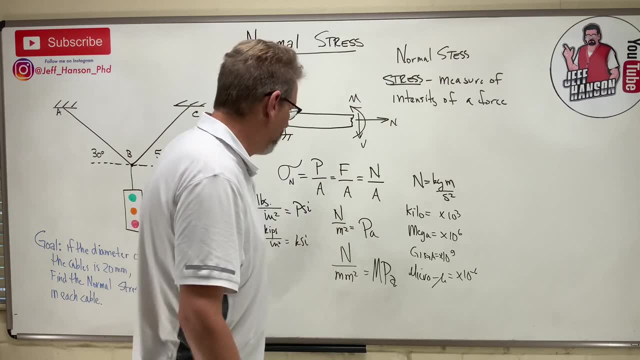 right And does this cancel out? And then I got to make sure I have the right number of decimals. It is so important. If you'll just do your units in your work, your grade point will go up a whole 10 points, I promise you. okay, Okay. so that's stress, normal stress, the intensity of the force. 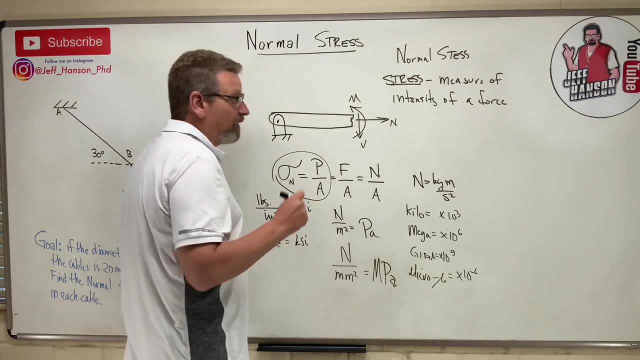 And this is the equation that we use right here. okay, So I'm going to put this over here because as we go along, I'm going to start adding equations over here. I'm going to kind of keep a little running equation sheet that we're using in here. 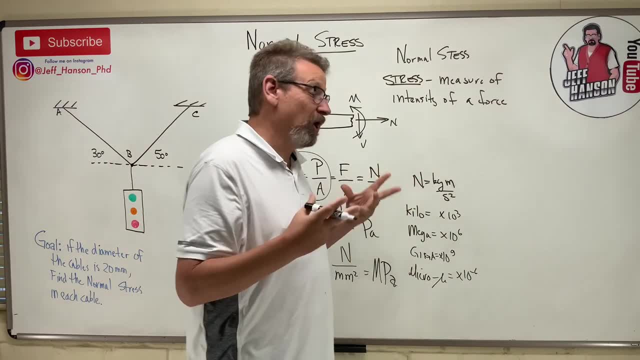 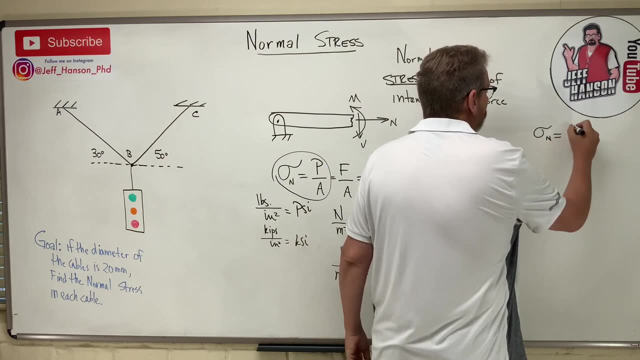 in solids, because in statics we made up our own equations. but in solids there are a lot of equations, And so this is going to be our first one. Sigma normal is equal to P over A. okay, So there's equation number one, and that is normal stress. 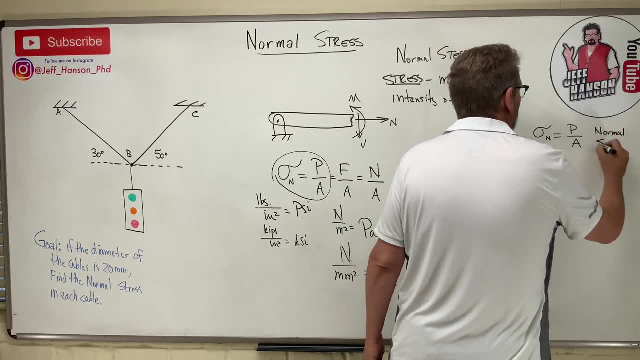 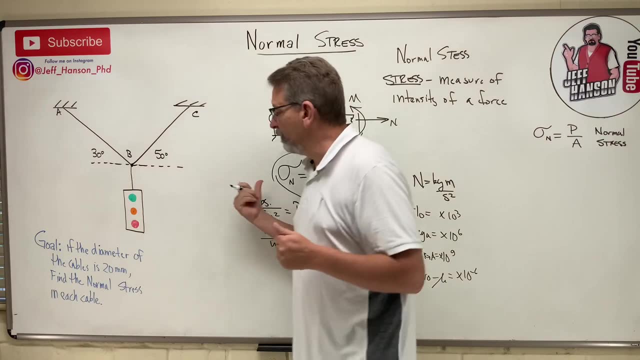 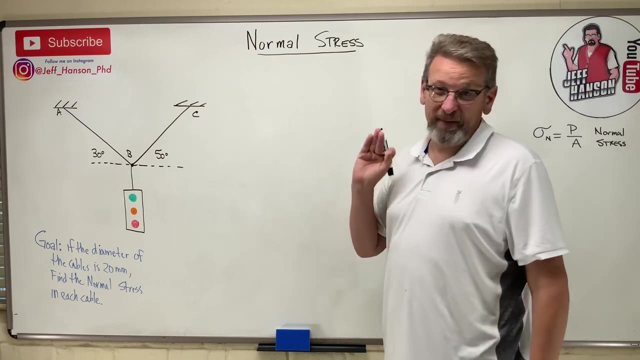 okay, All right, so let me erase this. and I have a little problem for us to use our normal stress on right there. Let me erase this. Okay, so this problem says: if the diameter of the cables is 20 millimeters, find the normal stress in each cable. You know what that looks like That looks. 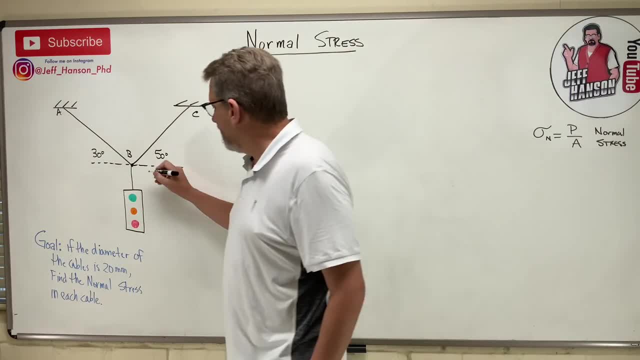 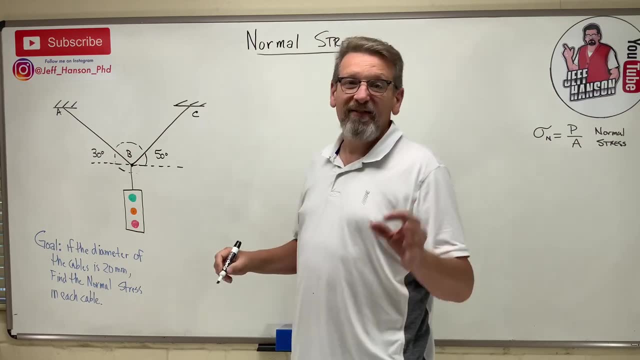 like a statics problem, doesn't it? That looks like if I went in and I did a free body diagram on joint B there, I might be able to figure that out, And that's exactly what you have to do. That's why statics is so important, because 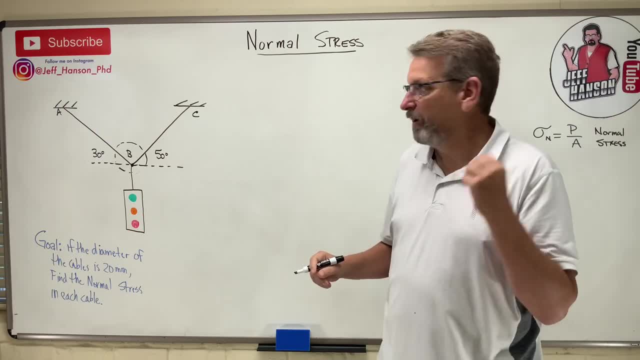 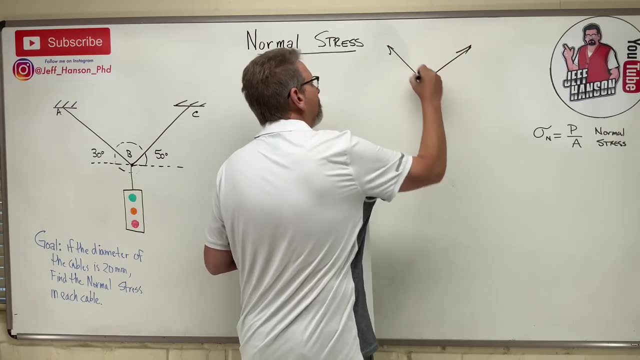 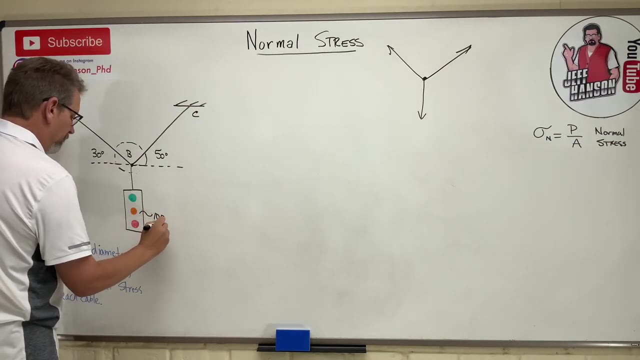 every solids problem starts off with a statics problem. every one of them, okay. So here we go, Let's go up here- Here's that joint B- And let's say that the light, the light is 100 newtons. okay, 100 newtons. 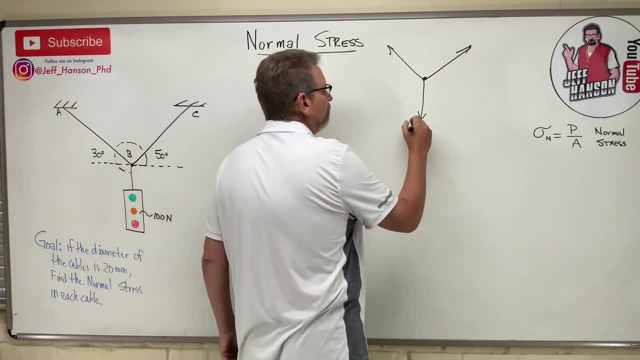 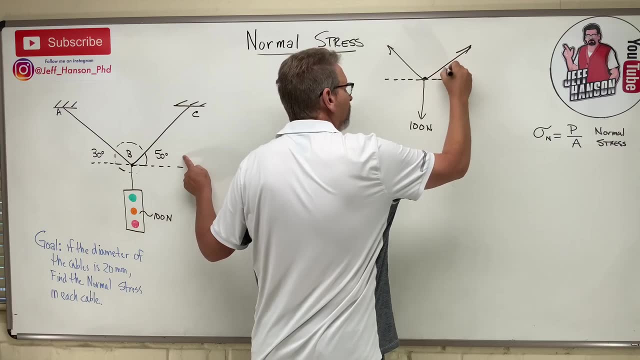 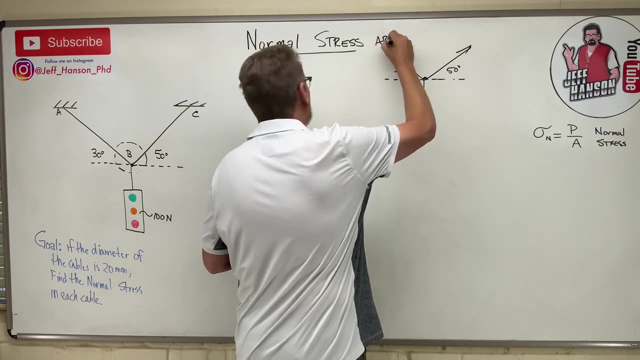 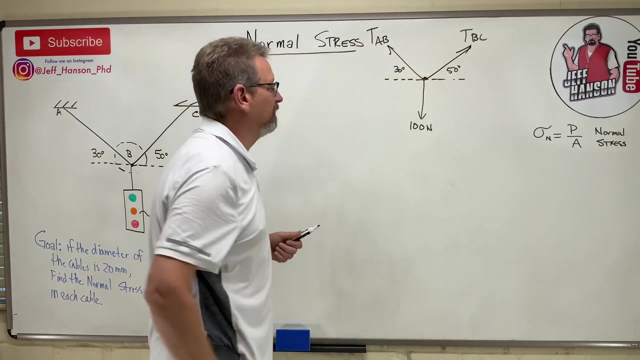 So what do we have over here? We have 100 newtons And we have- what is this guy? 50 degrees and 30 degrees, And we'll call this guy what? AB? And this guy is BC. Okay, I'm going to put a T for tension, okay, And then let's break those. 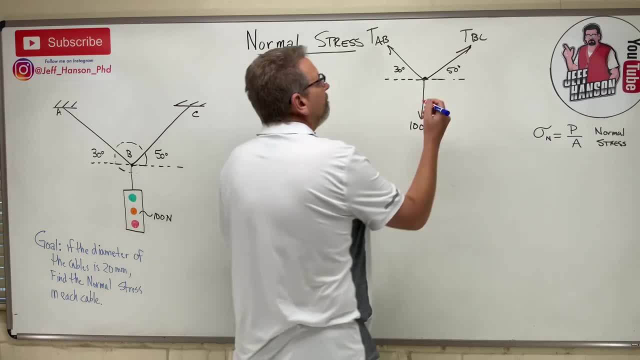 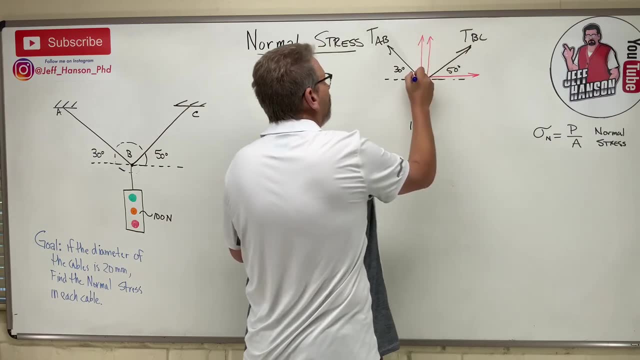 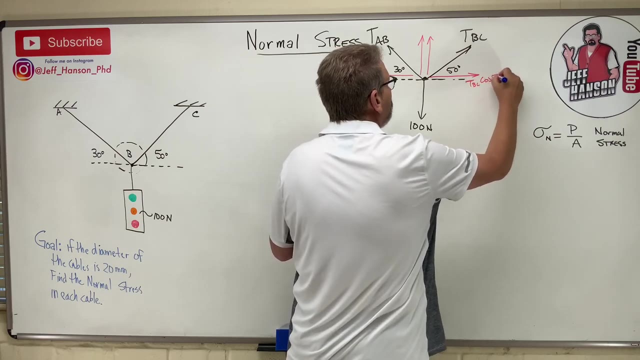 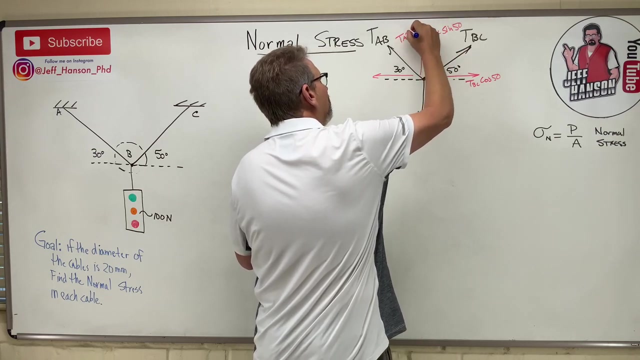 two vectors into components. I got my red pen somewhere here. Okay, so one component there, one component there. This guy has two components as well, And this is TBC cos 50,, TBC sine 50,, TAB sine 30, and TAB. 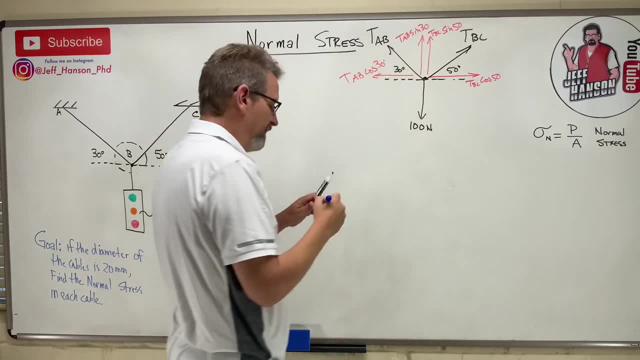 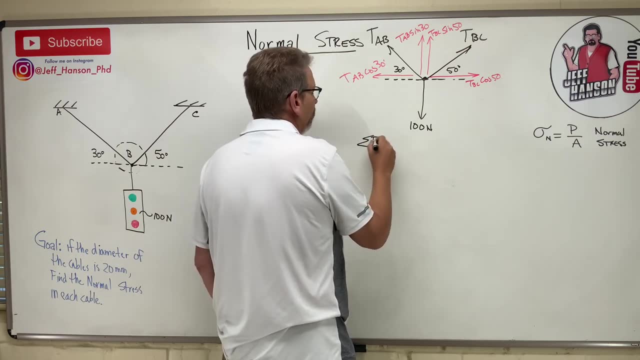 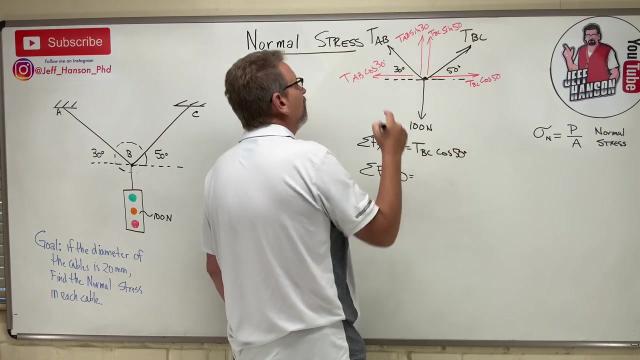 cos 30.. Okay, there's everything broken into components, So I should be able to write my equations: Some of the forces in the X, some of the forces in the Y. Okay, here we go In the X direction. I've got TBC- cos 50.. And what else do I have? Minus TAB, cos 30.. 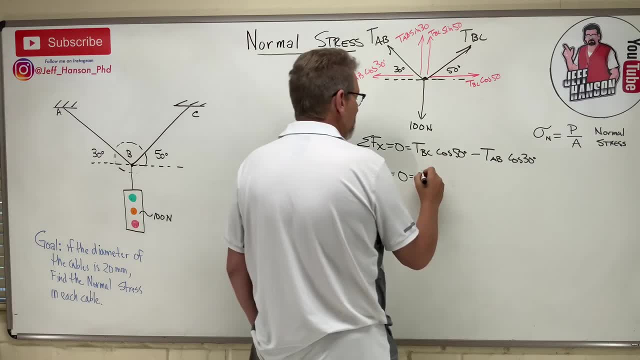 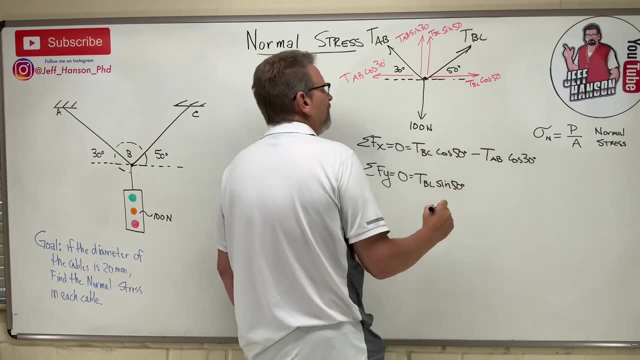 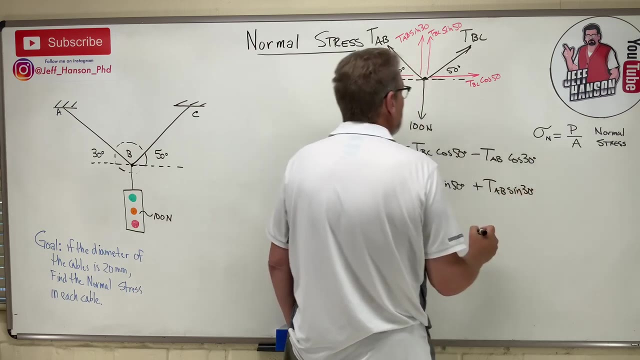 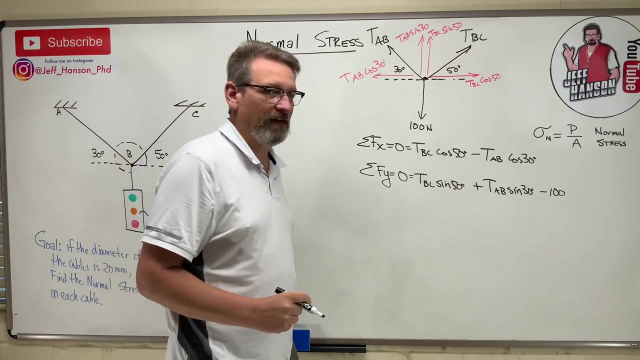 And in the Y direction, I've got TBC sine 50. And then I've got TAB sine 30. And then I have minus 100.. Okay, let me get my calculator. This looks like we can simplify this, All right. so I got cosine of 50, which is 0.643.. 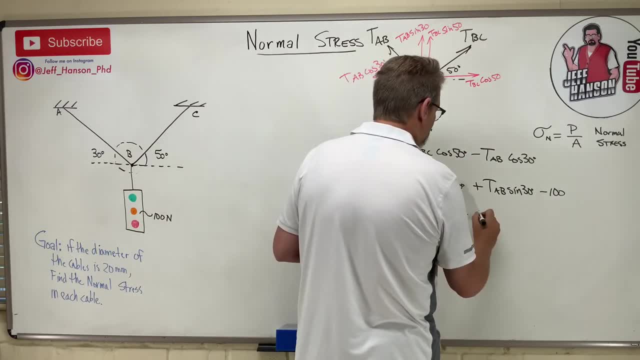 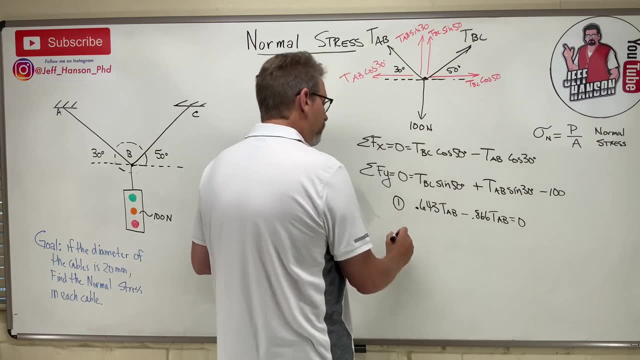 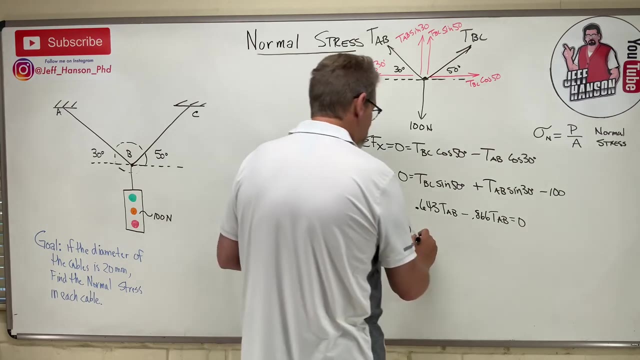 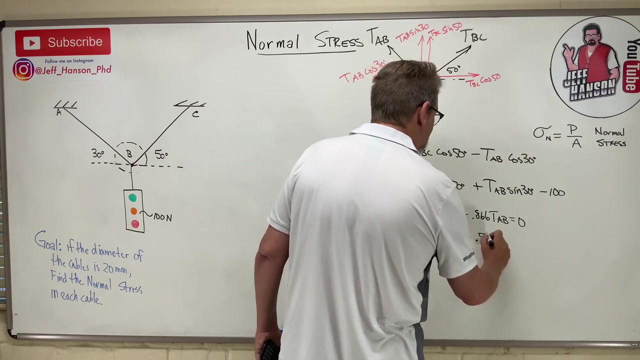 And then the cosine of 30 is 0.643.. And I've got cosine of 50,, which is 0.866.. All right, so I've got TBC sine 50, which is 0.866.. And then I've got cosine of 50,, which is 0.866.. 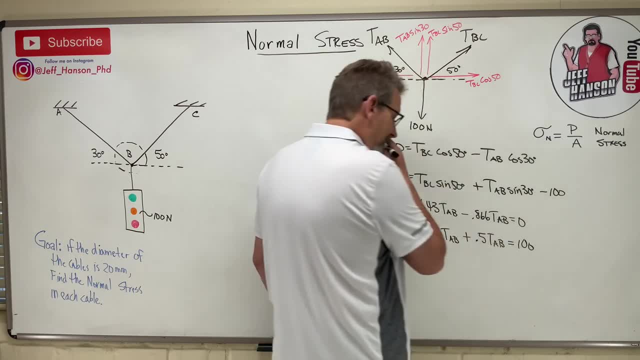 There's equation number one, And equation number two is the sine of 50, 0.766, .5. TAB equals 100.. So there's two equations, two unknowns And I've got a little handy-dandy system solver here. Let's see if we can get this. And then I've got cosine of 50, which is 0.866.. And then I've got cosine of 50, which is 0.866.. And then I've got cosine of 50, which is 0.766.. 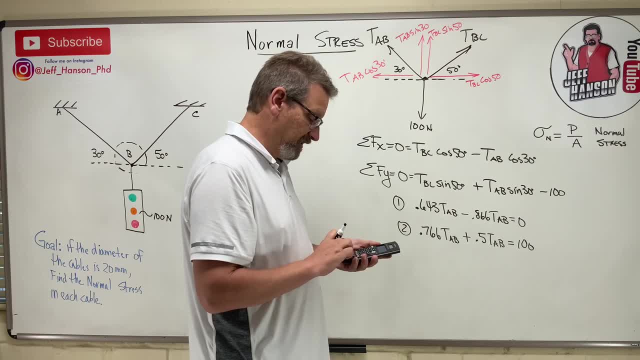 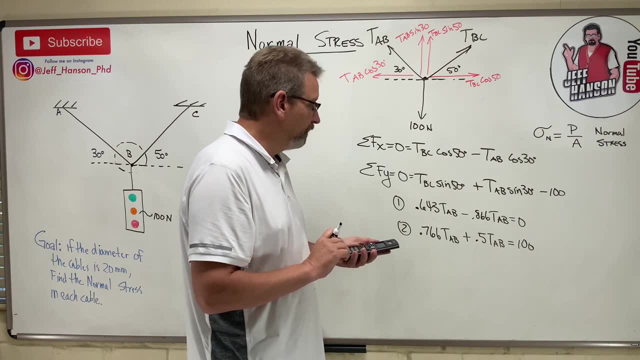 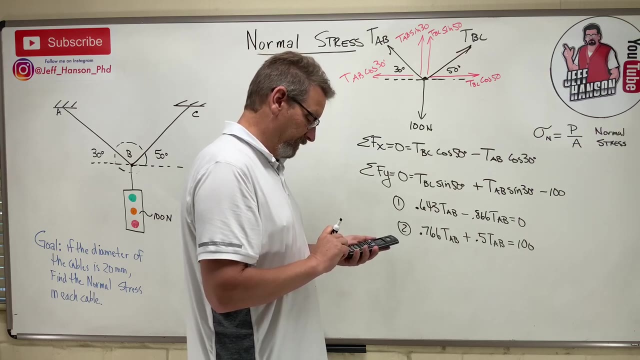 this, Here we go. We got 0.643.. Enter Negative: 0.866.. Enter: Zero Enter. If y'all haven't learned how to use this system solver on your calculator yet, you are missing out 0.5100.. And this is an. 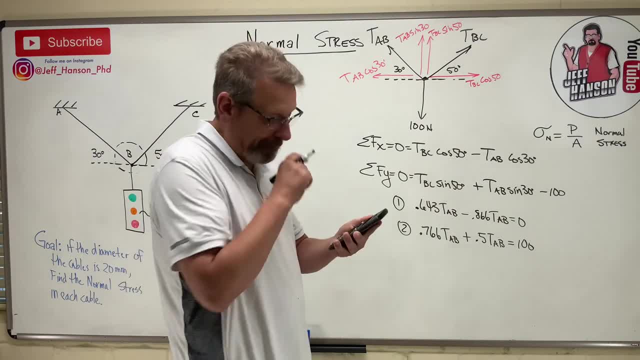 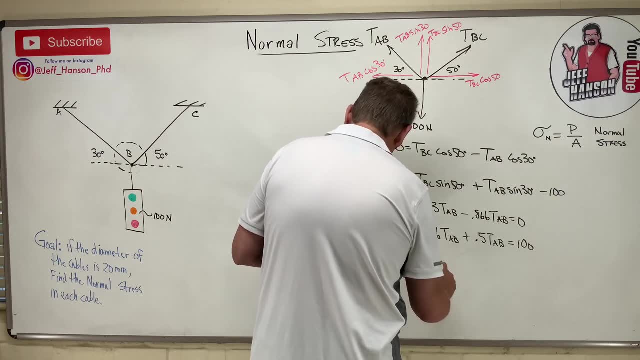 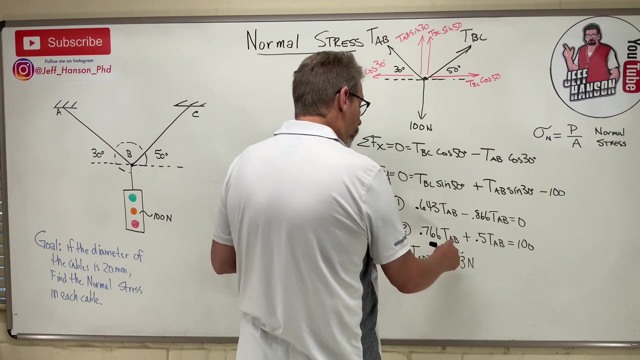 FE-approved calculator. It's the TI-36 Pro. Okay, And it tells me that TAB is 87.93.. And T? what is the other one? Oh, I did that wrong. No, This is not AB, That's BC. 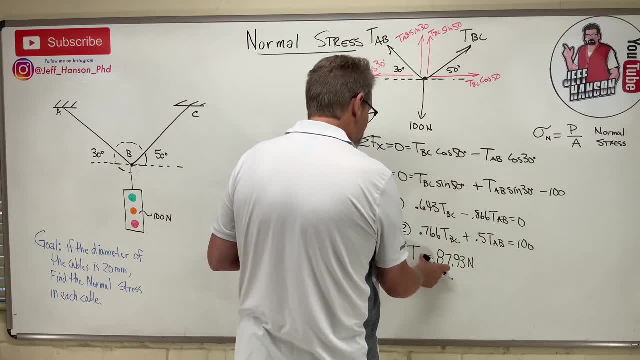 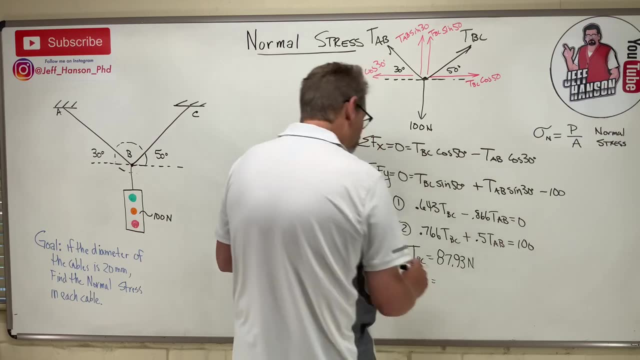 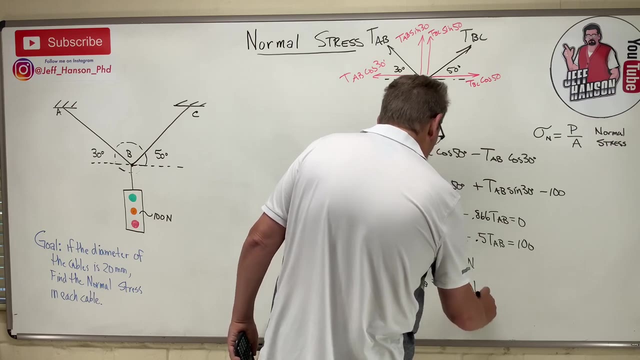 This is BC. I bet y'all were going. what are you doing? What are you doing? I got it, I got it, I got it, We're all good. And the next one is 65.3.. So now I use statics to find the tensions in the 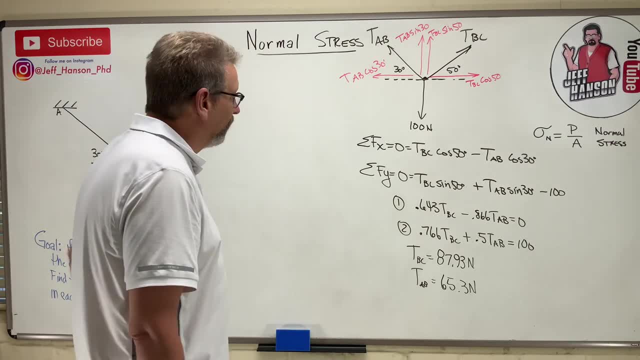 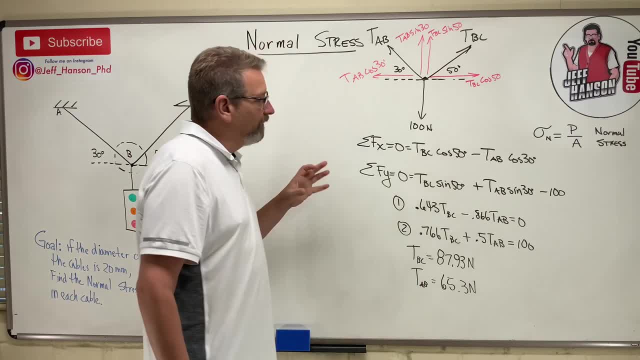 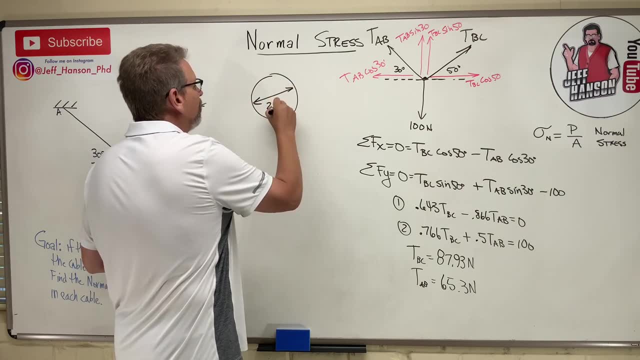 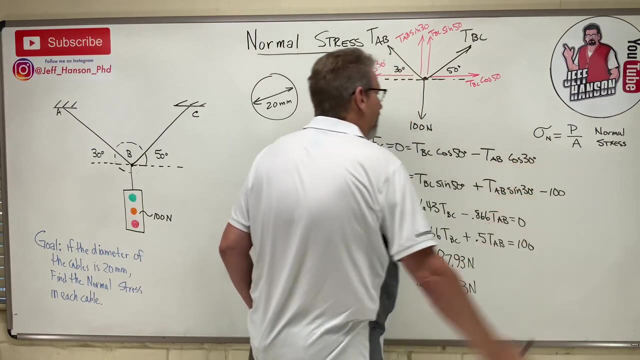 each one of the cables with a 20 millimeter diameter. So one of the things- other things I need to do is blow this up. Here's the cable. The cable has a diameter of 20 millimeters, which means it has a cross sectional area. That's what that is right there, That A. 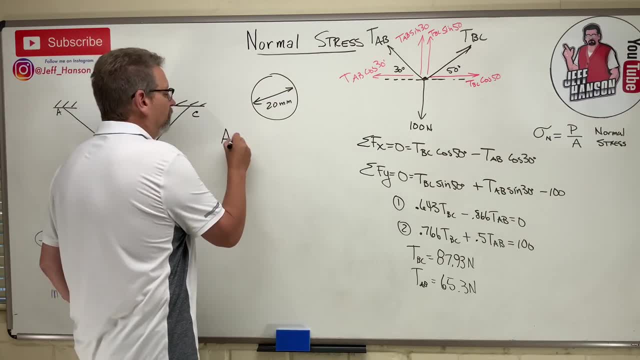 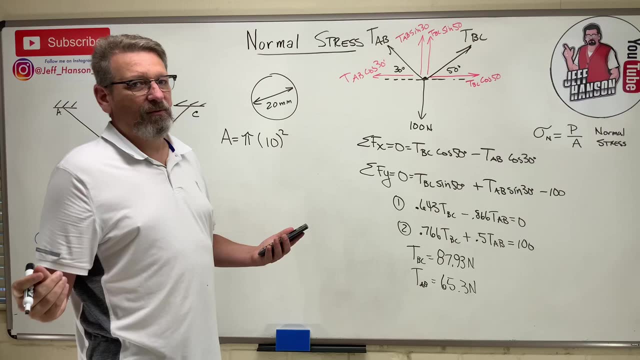 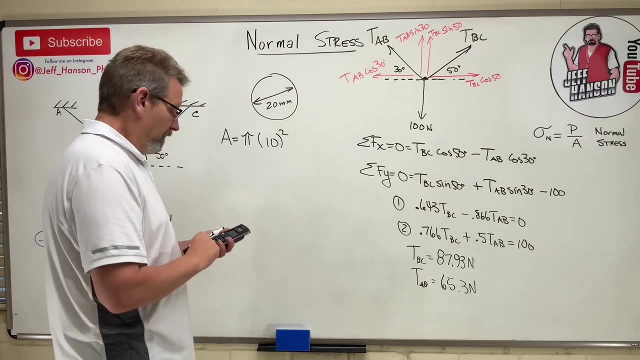 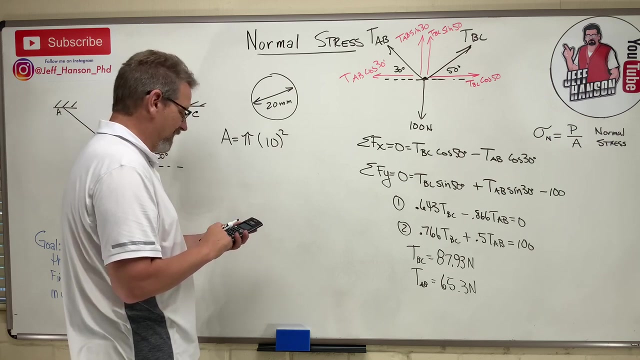 is the cross sectional area, right? So the area is equal to pi R squared. Y'all ever wonder why pi R squared and K cake are round? No, wait a minute. Pi are round and cake are square. Okay, Math joke, Math joke. A bad math joke, but it's a math joke, Okay. So pi, that's times 100,. 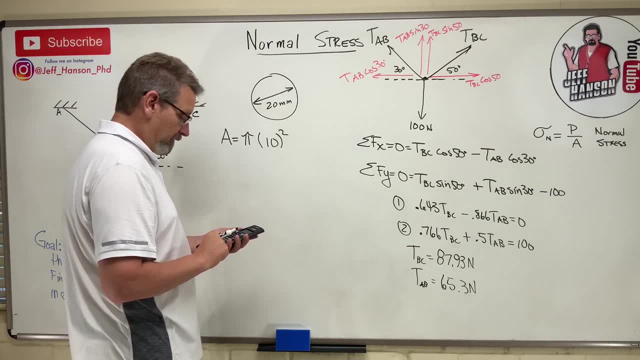 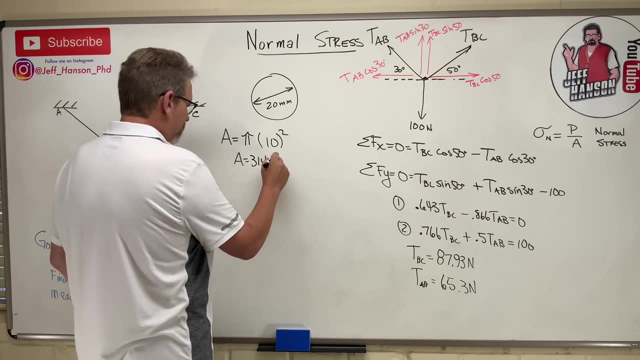 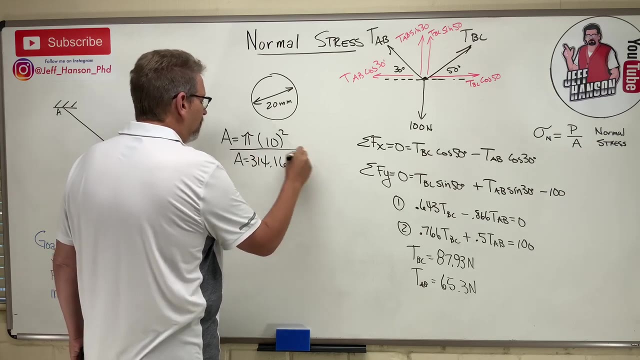 isn't it? Okay, We know what that is, don't we? Area is equal to 314.16,, of course, and that is millimeters squared, Okay. So we needed that for our next equation. So here we go, Sigma. 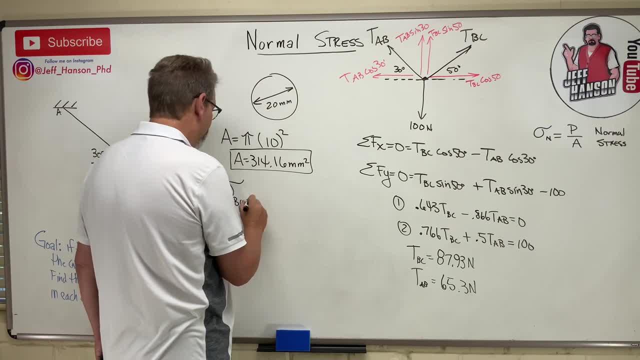 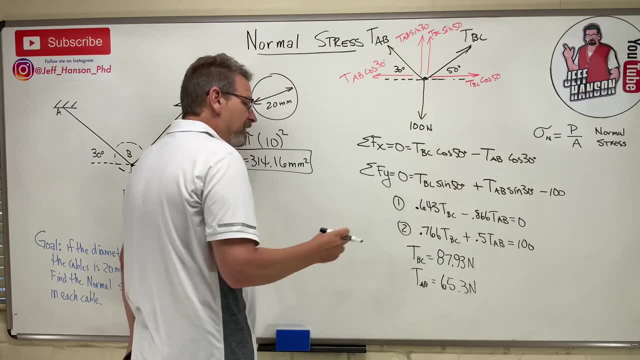 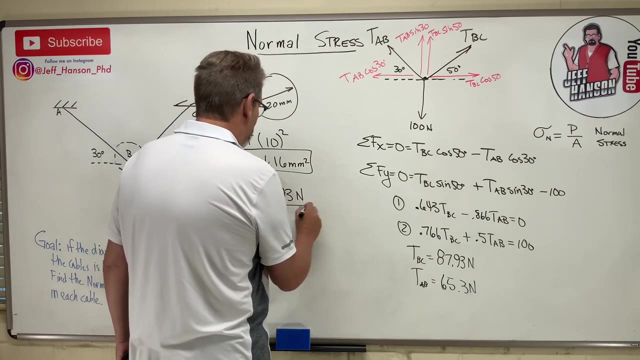 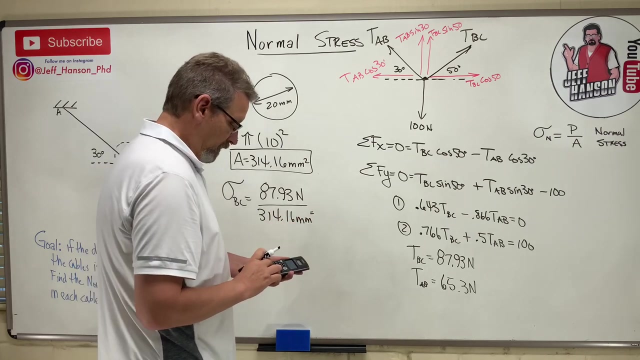 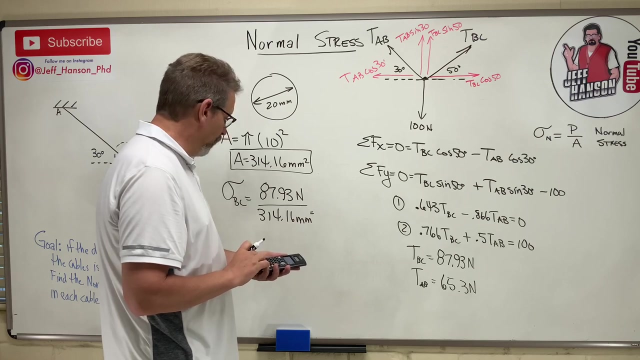 sigma BC. Okay, The normal stress in cable BC is pretty easy. It's just force over area. Okay, And the force, we've got that 87.93.. And that's newtons divided by 314.1.. 0.16 millimeters, which is equal to I don't know. 87.93 divided by 314.16 is equal to 0.279. 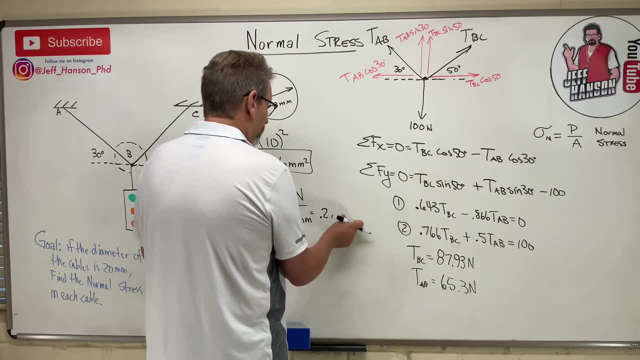 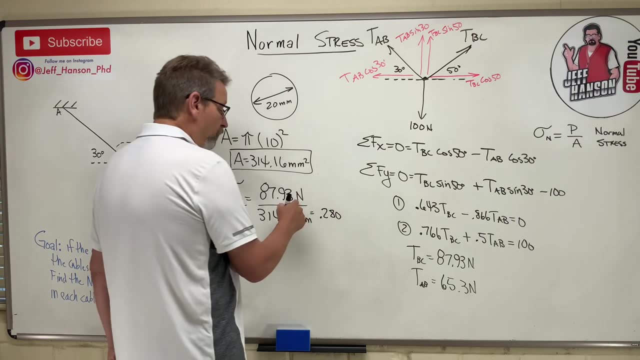 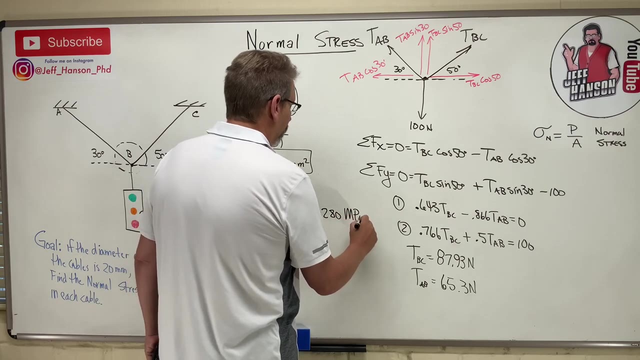 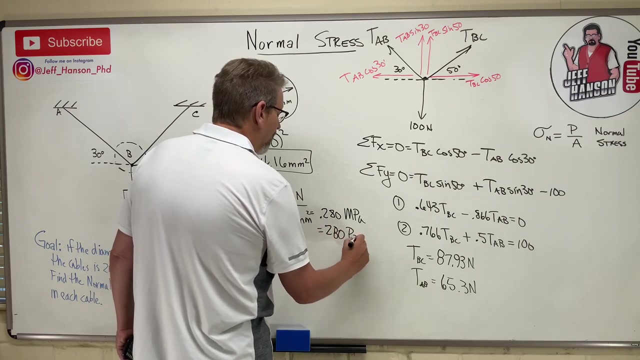 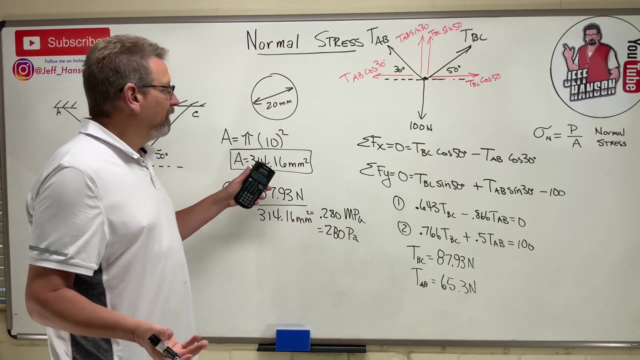 Eight, which is really 0.28, isn't it Okay? And that is what is that? That's newtons over millimeters squared, which is- we just did that- megapascals, right? Or you could write that as 280 pascals, Okay, Now, yes, that cable is way.